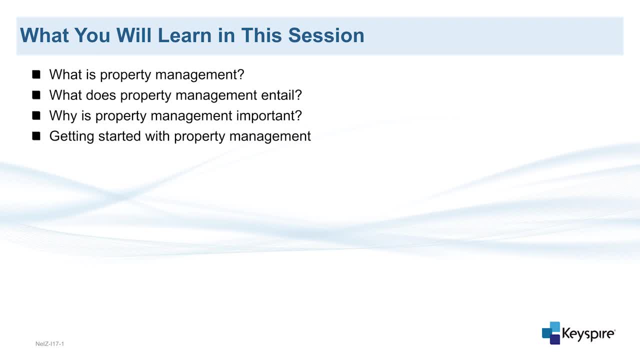 explore some of the ways to get started with managing your own properties. Some of the key terms you'll hear in this session include property management: an individual or company responsible for the day-to-day functioning of a piece of real estate. Landlord-tenant law. 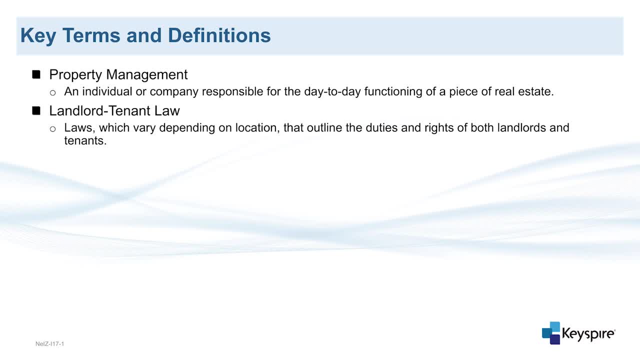 laws, which vary depending on location, that outline the duties and rights of both landlords and tenants. Lease: a written agreement between an owner and a tenant under which the owner allows the tenant the right of exclusive use of the property for a specified time, rent and terms. 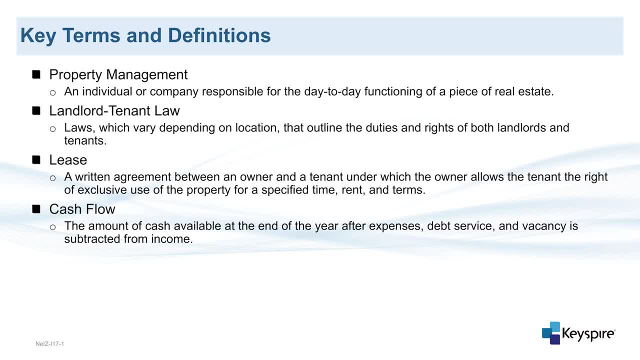 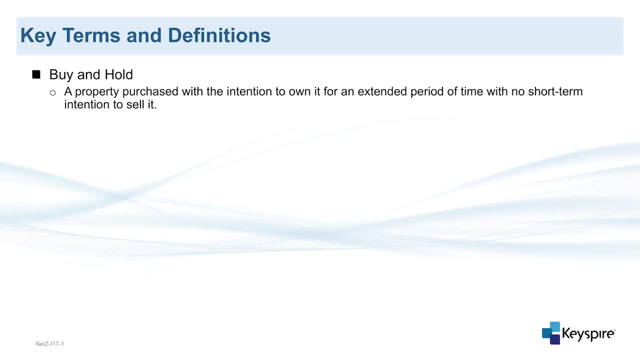 Cash Cash flow. The amount of cash available at the end of the year after expenses, debt service and vacancy is subtracted from income Vacancy. Available rental units that are vacant or unoccupied. Buy and hold A property purchased with the intention to own it for an extended. 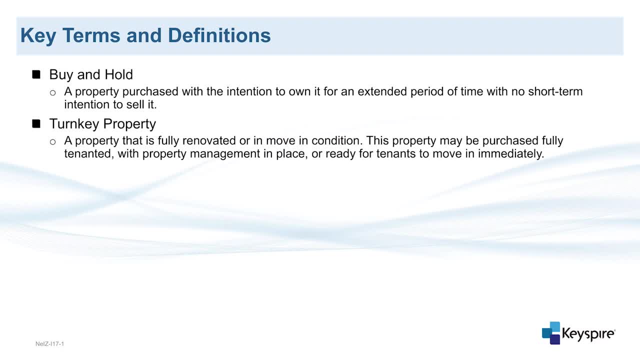 period of time with no short-term intention to sell Turnkey property, A property that is fully renovated or in move-in condition. This property may be purchased fully tenanted, with property management in place. Return on investment or ROI: The measurement of return on an investment relative to the capital. 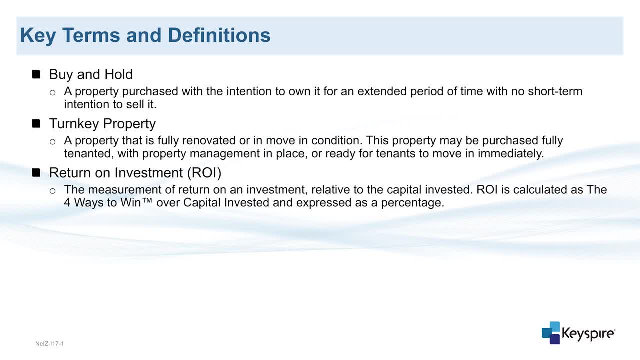 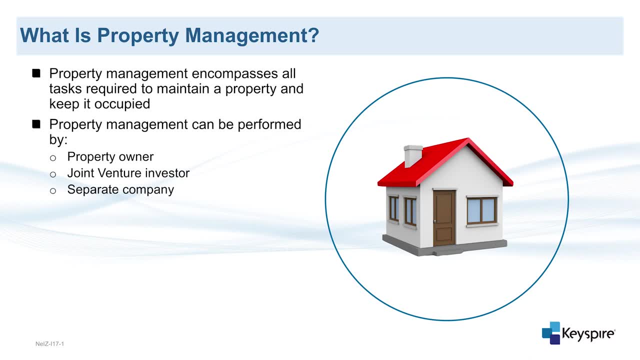 invested. ROI is calculated as the four ways to win over capital invested and expressed as a percentage. So what is property management exactly? Property management, whether performed by yourself, a joint venture investor or a separate company you hire to manage your investment property. 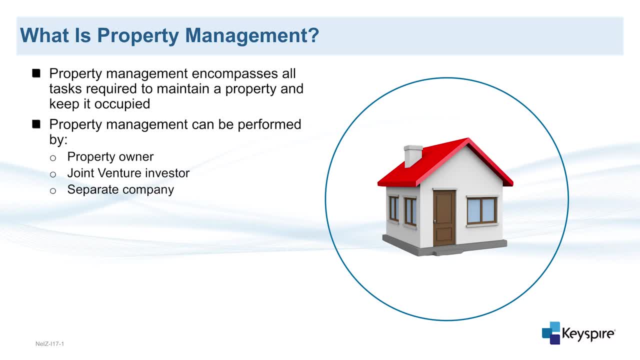 encompasses all tasks requires to maintain the property and keep it occupied, Regardless of who is actually managing the property. property management includes a number of responsibilities that you, as an investor, should be aware of. Let's briefly introduce these various responsibilities, which include, but are: 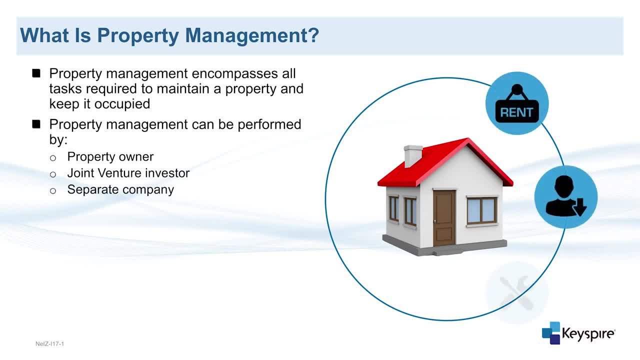 not limited to rent tenants, maintenance and repairs, knowledge of the landlord-tenant law, supervising and managing the budget and taxes. Future sessions in this course will discuss property management responsibilities in the future. So let's get started. Property management responsibilities. 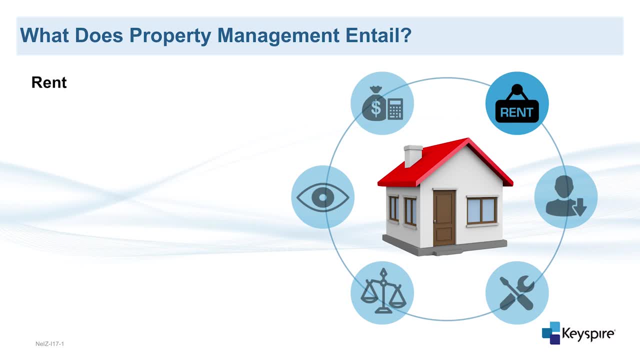 The first major responsibility we're going to discuss is rent, including setting rent, collecting rent and adjusting rent as necessary Depending on the specific situation. the rent would be set by either the investor, the property manager, or the joint venture investor. From there, the property manager would be. 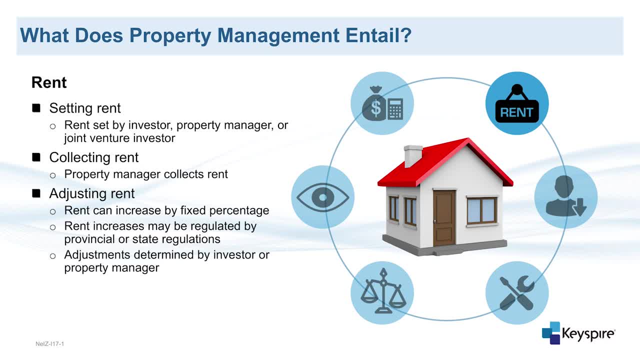 the one who collects the rent from the tenants. Each year, the rent can be increased by a fixed percentage, depending on state, provincial or municipal laws. Again, any increases or decreases to rent is determined by either the property manager or the investor, depending on the situation. Another major area of responsibility for property managers: 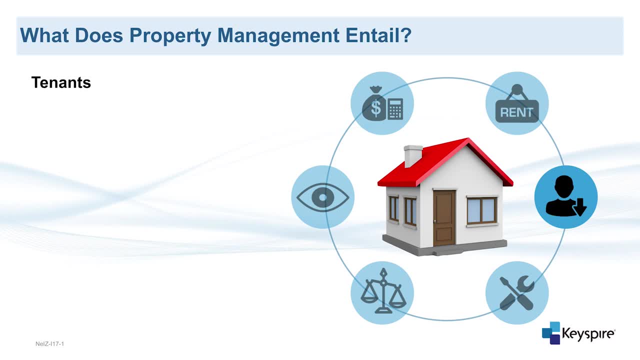 revolves around managing tenants, which itself has a number of responsibilities: Property managers must find good applicants, screen those applicants, select the perfect tenants, handle leases, handle complaints and emergencies and finally handle move-outs or evictions. We'll discuss these in more detail in various sessions of this course. 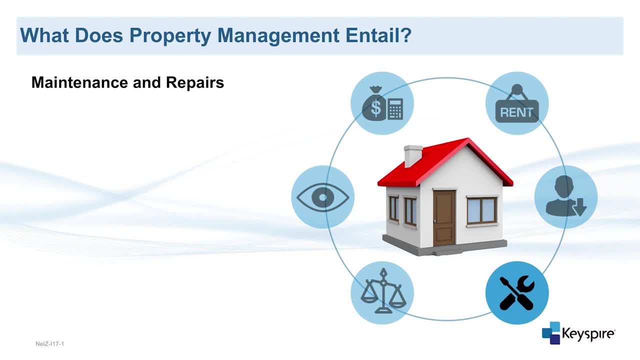 Property managers are also in charge of the physical management of the property, including day-to-day maintenance as well as repairs. Day-to-day maintenance tasks could include landscaping duties, snow removal and trash removal, to name a few. If an issue arises and requires repair, it's also the property manager's responsibility to fix any problems. 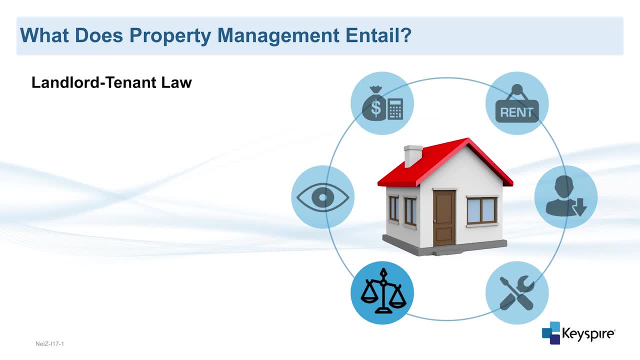 Since the property manager is dealing so closely with the tenants on a frequent basis, it's vital for the property manager to have a full understanding of the landlord-tenant law for the area the property is in. There are various state, provincial and municipal laws regarding the. 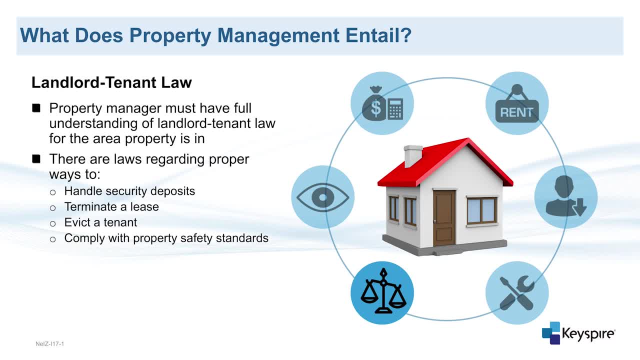 proper ways to screen a tenant, handle security deposits, terminate a lease, evict a tenant and comply with property safety standards, to name a few. To maintain a cash-flowing property, these laws must be understood and followed. In some situations, property managers are also. 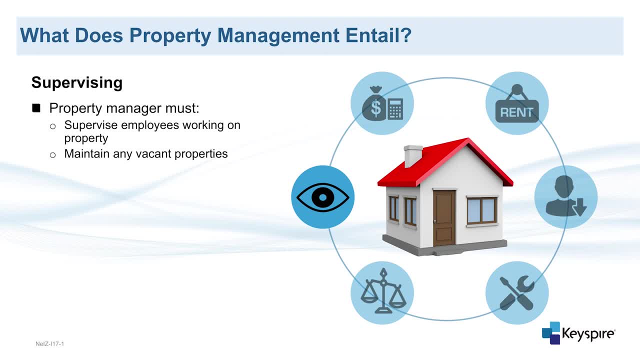 responsible for supervising employees' working in the property and for supervising vacant properties. If there are employees working on the property, such as concierge or security personnel, the property manager must maintain and manage these relationships. Additionally, property managers must ensure that any vacant properties under their management are routinely maintained. 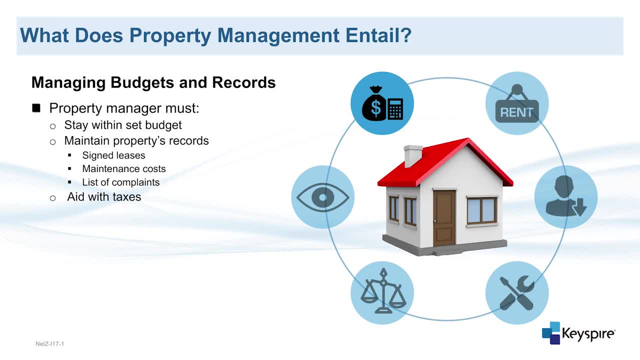 Property managers are also responsible for staying within the set budget for the property and for maintaining the property's records, such as signed leases, maintenance costs and list of complaints. Finally, property managers can either help owners file their taxes or, alternatively, be endowed with the power to file the taxes on behalf of the owner. 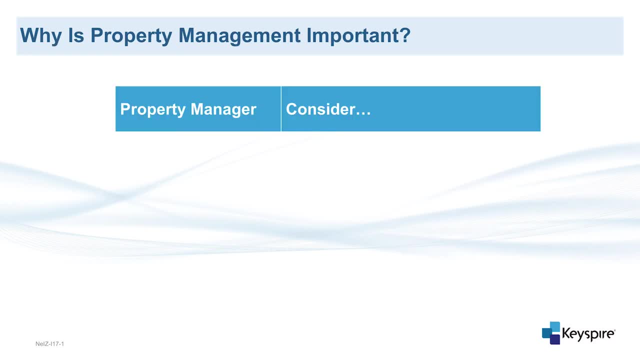 unless, of course, the property manager is also the owner. With so many crucial responsibilities falling under property management, it's easy to see why it's so important. Your main goal as a real estate investor is to receive a return on your investment and build your wealth Well. 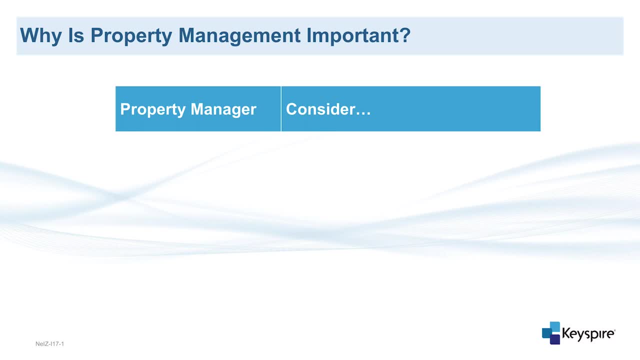 unless your investment properties are rented out to tenants and you have no vacancies, you won't be able to see cash flow. If you decide to manage your own properties, you'll have to consider the cost of your time If you are going to work with a joint venture investor. 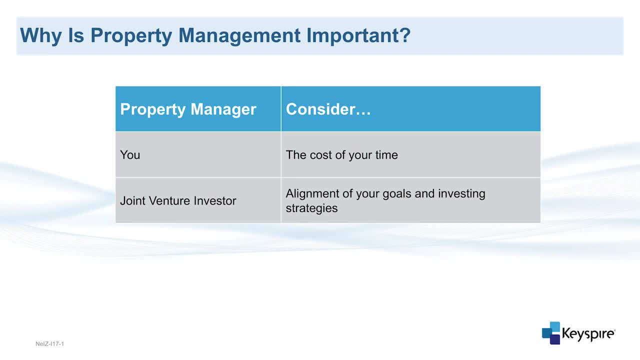 you will want to consider alignment of your goals and investment strategies. If you're going to hire a third-party company, you will want to consider the financial cost and management of the property manager. As you can see, regardless of your decision, property management comes with some important considerations. Your final decision will be determined by the 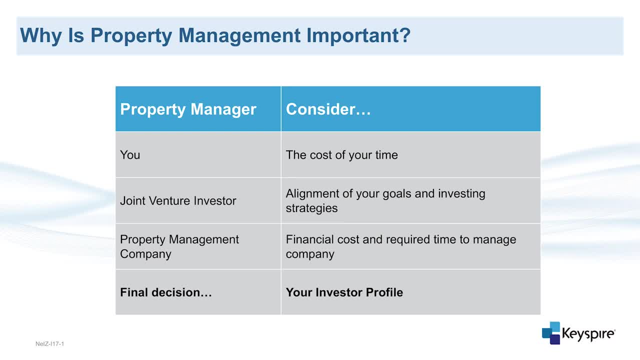 specific investor profile you have Keep in mind. the cost of time or money for property management is one that should not be skimped on. Savvy investors understand good property management can make the difference between successful investors and those who leave the business because of poor experiences. Ultimately, to build your wealth through real estate investing in rental. 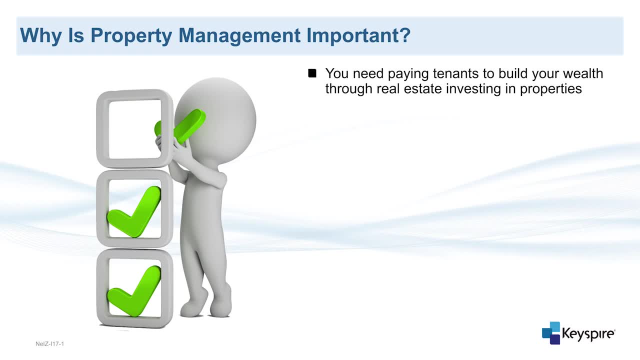 properties. you need to have paying tenants renting your investment properties. To manage a successful portfolio of property management, you need to have paid tenants renting your investment properties. of investment properties, you or your property manager need to complete a long list of critical tasks to ensure your property is fully tenanted, avoid vacancy or non-payment of rent, ensure the 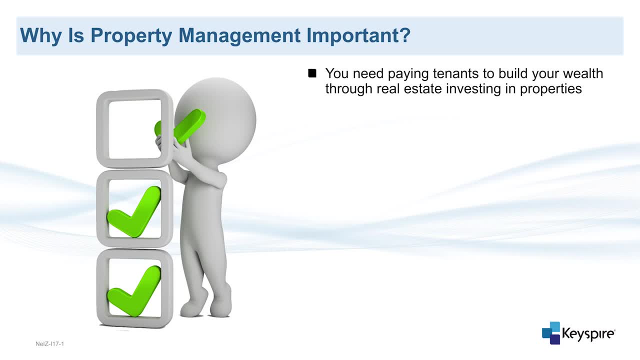 property is maintained and operating efficiently, and work to make management scalable so your portfolio can continue to grow and grow. This brings us to our main point. Property management is important because it puts well-qualified, paying tenants in your properties, it ensures efficient day-to-day operation and it provides overall continued maintenance to your portfolio. 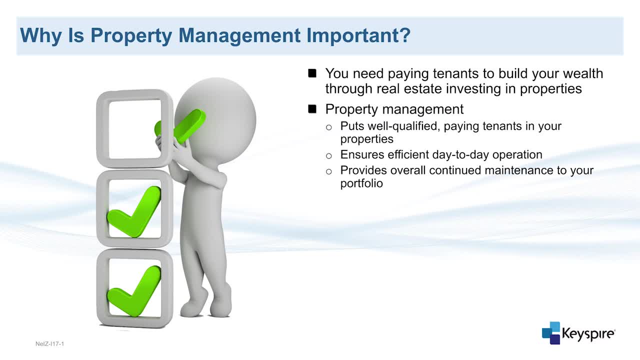 Solid property management can be the key to long-term wealth because once you obtain the investment, you want to ensure it continues to produce ROI as you originally projected. If you are not yet sure if managing an investment property is right for you, you do have the option of starting small. 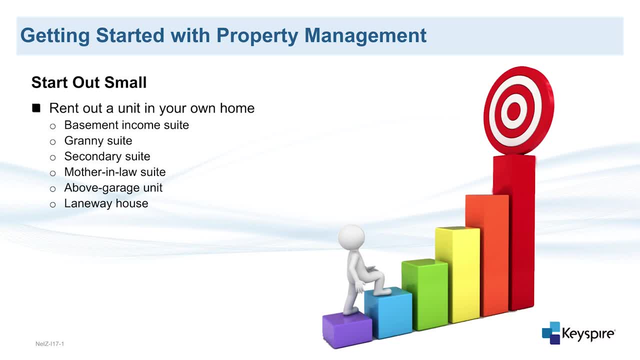 If possible, you can begin with renting out a unit in your own home. You may have a property with a basement income suite or a basement with the opportunity to add a legal income suite. Some properties have granny suites, a secondary suite or a mother-in-law unit. 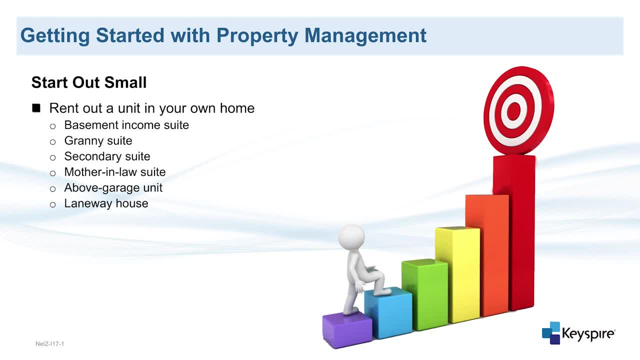 These can include an above-garage unit, a laneway house or an additional structure on the property. If you own one of these or have the option to add one, you can begin managing a rental property on a smaller scale. This will provide you with some extra income. 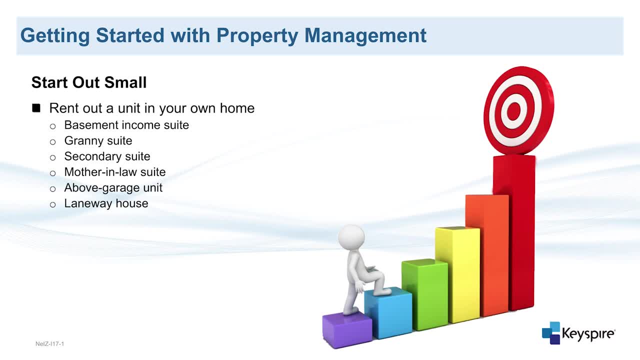 And allow you the opportunity to see if you like being a landlord. Of course, some people are not comfortable with the thought of strangers living in their homes, so you will want to assess your comfort level. Some potential landlords choose to rent to friends or family if the unit is on the same. 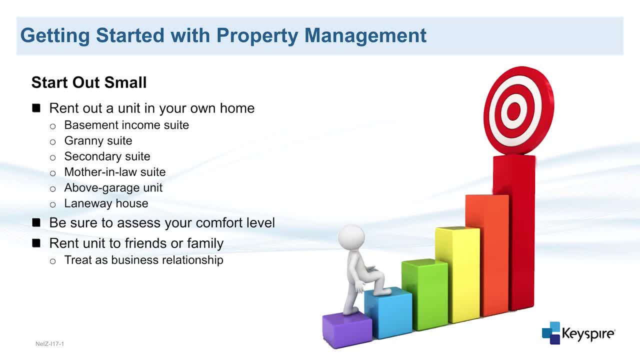 property as their main residence. This may give you a greater sense of security, but always remember that this is a business relationship. Be sure you are comfortable talking about money, can agree upon lease terms and writing, and that you won't have to worry about the cost of renting a property. 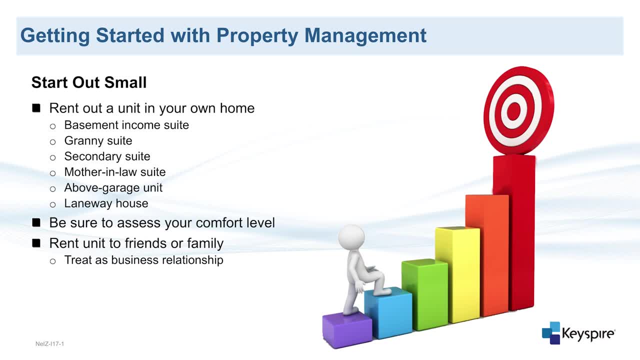 You won't have to chase them each month for the rent. If you are renting to friends or family, you also want to make sure you are very clear about each other's privacy and the terms of the lease. Think about what could happen if one of you 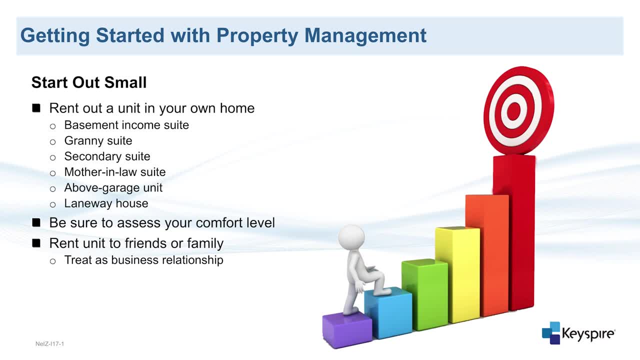 wanted to end the landlord-tenant relationship, You may discover that property management is not for you, and you don't want to be known as the one who kicked out Aunt Sally. Finally, if you do choose to convert part of your residence to a rental unit, 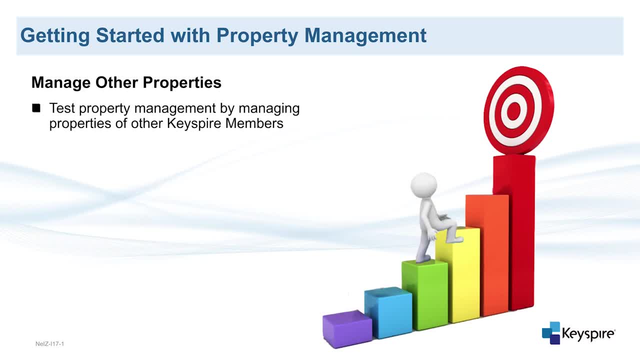 be sure it meets all zoning laws for your area. Alternatively, you may decide to test out property management by managing properties of other key spire members. Property management is a relatively low-cost way to get into real estate investing. It requires time, organization, customer service skills and an understanding of local regulations. 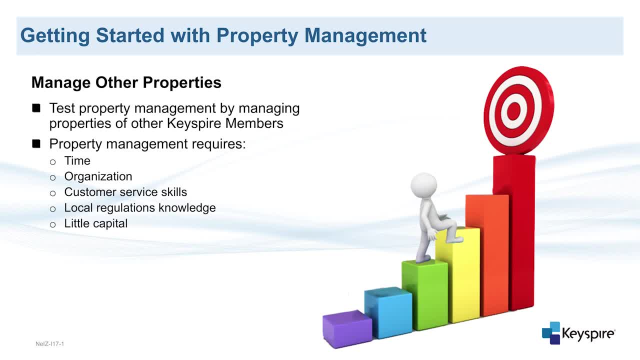 but it doesn't require a lot of capital, So it's a great earned income strategy for those who can't afford to purchase a property themselves. yet Since some investors choose to invest in properties that are far away from their primary residential location, they may decide to test out property management by managing properties of other key spire members. 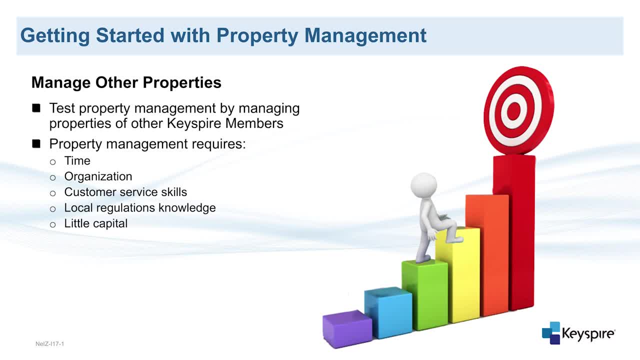 They may decide to invest in properties that are far away from their primary residential location. They would need to hire property managers to manage their investment properties. Take advantage of your key spire network and seek out opportunities where you can manage properties, perhaps even on a part-time basis, for members who are investing from afar. 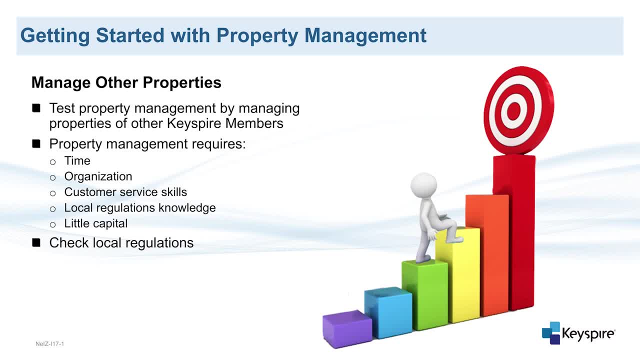 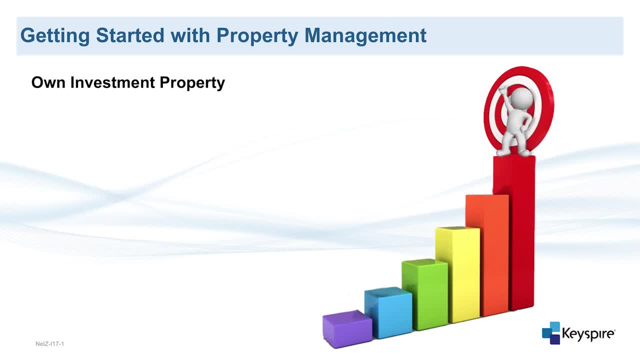 Just be sure to check local regulations, as some states and provinces require licenses for property managers to manage other people's properties. Perhaps you want to keep your home and real estate investments separate, or perhaps you are not interested in investing in a property. You may decide to invest in a property that is not in your area. You may decide to invest in a property that is not in your area. You may decide to invest in a property that is not in your area. Perhaps you want to keep your home and real estate investments separate, or perhaps you are not interested in forming a joint venture with another investor. 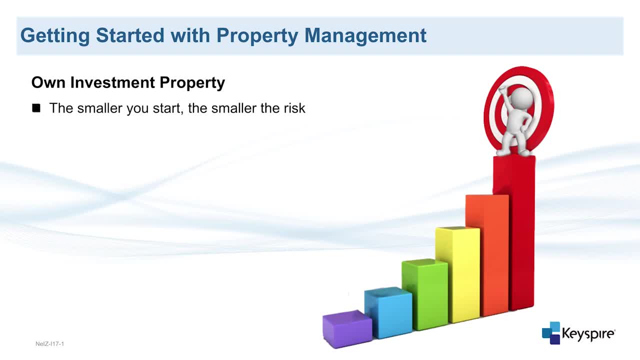 Instead, you may want to own an investment property. As with all investments, the smaller you start, the smaller the risk you take on. However, once you decide to take on more of an investment, you also exponentially increase your potential returns on that investment. 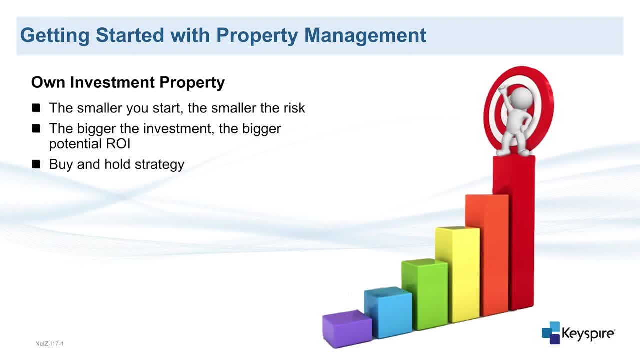 The real estate investment strategy we will be discussing here is mostly buy and hold, wherein you purchase the property, perform any repairs if necessary and then maintain that property as a positively cash-flowing investment. One strategy that you may choose to use for your first buy and hold is to purchase a turnkey property that is already tenant-occupied. 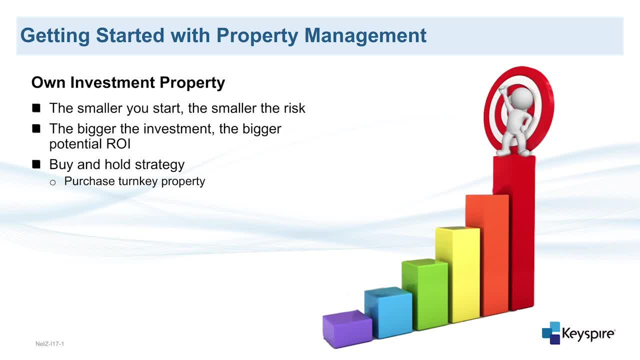 This means that the property is already rented and you just take over the lease. as the new owner, You start collecting the rent right away, so it is a very easy transition. However, remember that when you purchase a turnkey property, you are purchasing a property that has all of the work. 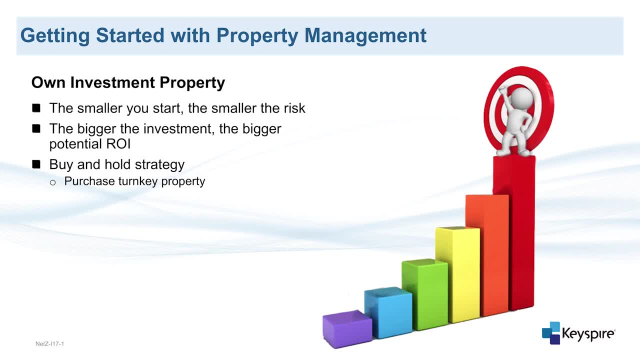 already done, So you won't have to perform renovations, advertise the property or screen tenants, which means less work for you, but you often pay more to purchase this type of property. As you gain experience as a real estate investor, you will most likely want to diversify your 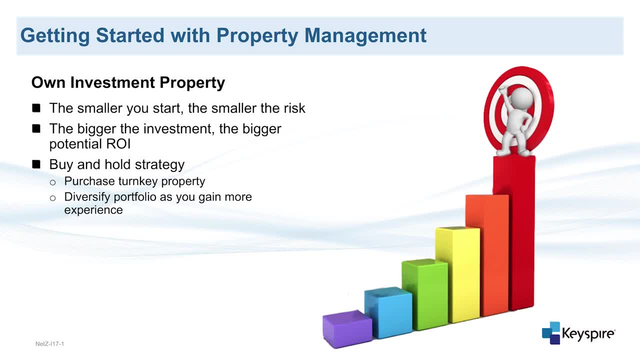 portfolio. You can then look at expanding into different types of rental properties, purchasing in different locations and or investing in different cash flow types. These can include properties requiring more renovations. You will be able to purchase them at a lower price, but you will also have to factor rehab. 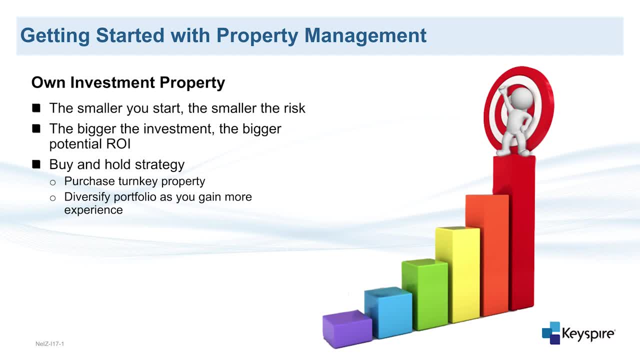 costs into your expenses Or purchasing underperforming properties, including those with potential for future expansion or development. This can also be a great investment to take on with a joint venture investor. In this strategy, you work with another investor who provides cash for the purchase credit to secure financing sweat equity for any necessary repairs or the 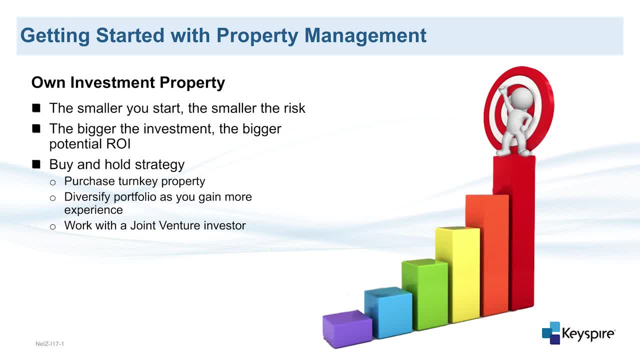 day-to-day property management or some combination of the two. You can also purchase a property that can be used as a joint venture investor. You then split the profits, which will reduce the amount you make on each individual deal, but allows you to do more deals. spread your investable capital. 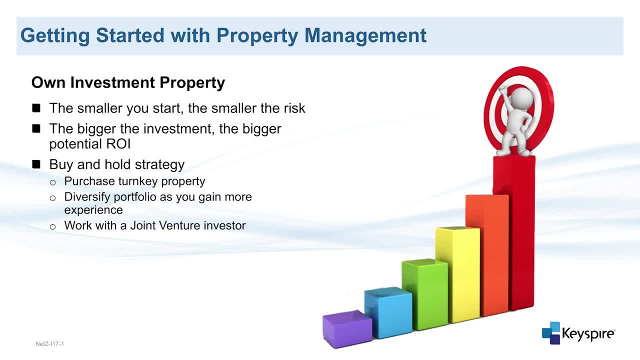 further and possibly make better investments overall. For more information on joint ventures, please see the Keyspire course devoted to joint ventures. When determining whether property management is right for you, be sure to assess your investor profile and your specific situation to make property management decisions that work for you. 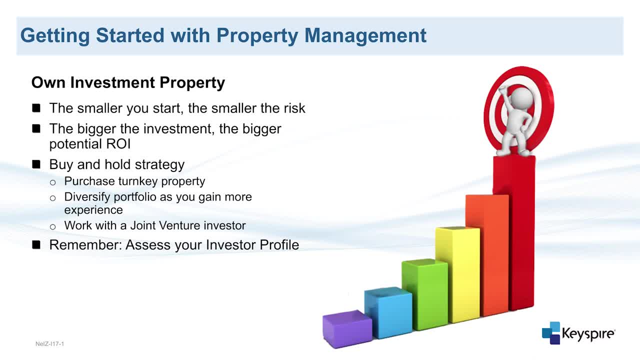 Remember. if you have any questions, please feel free to ask them in the comments below. You are building your real estate portfolio to increase your wealth and to do so, you need to determine what your time and money situations can allow. Refer to the: Determine Your Investor. 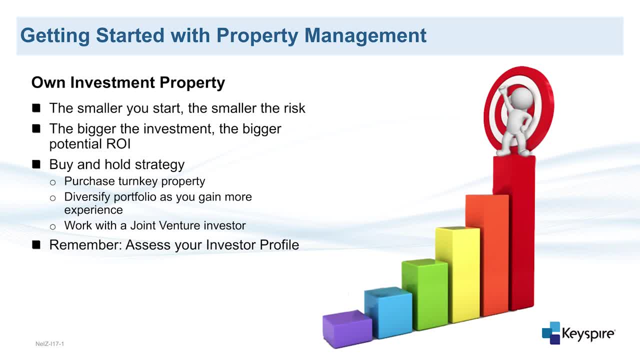 Profile course on the member dashboard for more information. Regardless of who is managing your property, which we will discuss in the Who Should Manage Your Property session of this course, make sure your property has positive cash flow and total return on investment that aligns with. 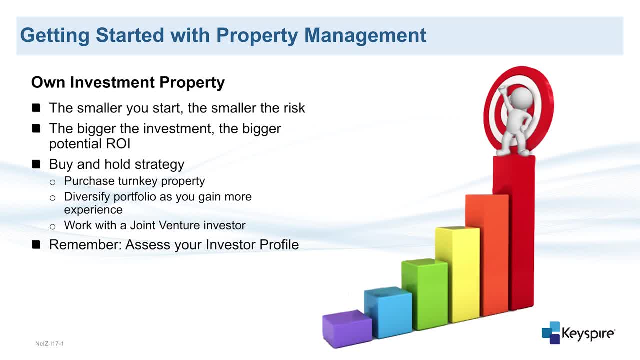 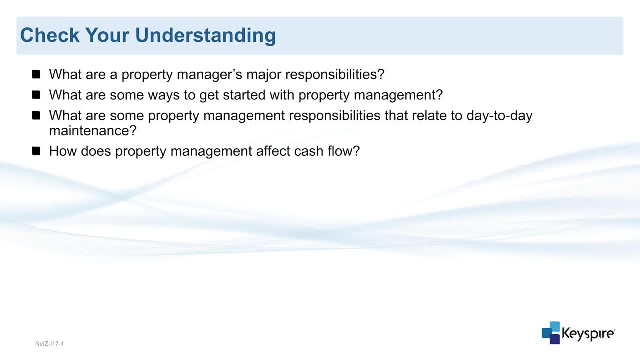 your investing goals. That is what will make it a strong real estate investor. Before we further explore property management, let's check your understanding of the basic concepts we've discussed so far. What are a property manager's major responsibilities? What are some ways to get started with property management? What are some property management? 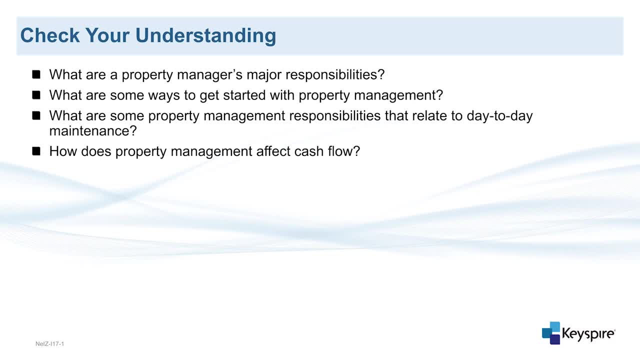 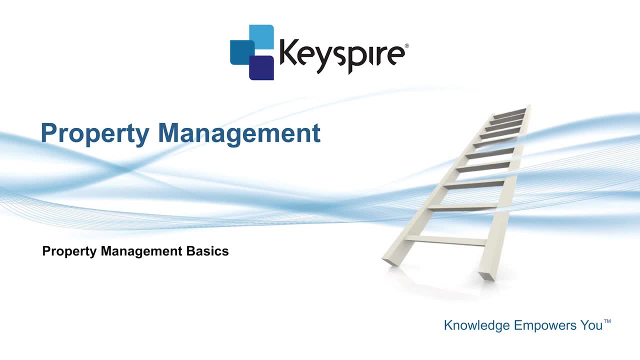 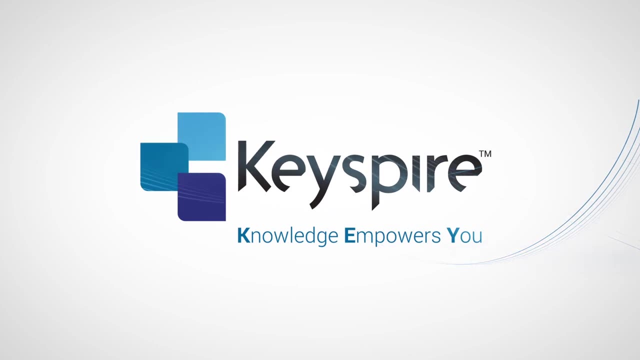 responsibilities that relate to day-to-day maintenance. How does property management affect cash flow? This concludes the Property Management Basics session of the Property Management course. Thank you very much for joining us today and we'll see you next time.